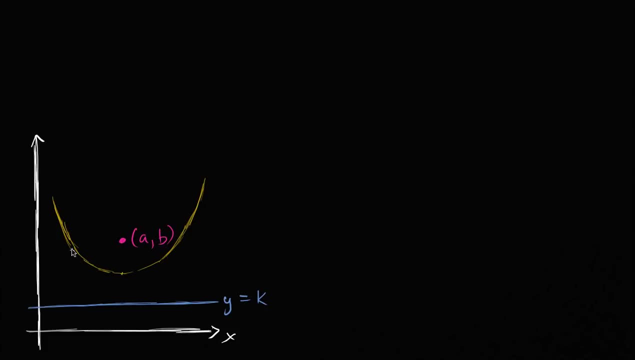 So let's do that. So let's take a arbitrary point on the parabola. Let's say, we take this point right over here and its x-coordinate is x and its y-coordinate is y And, by definition, in order for this to be a parabola, 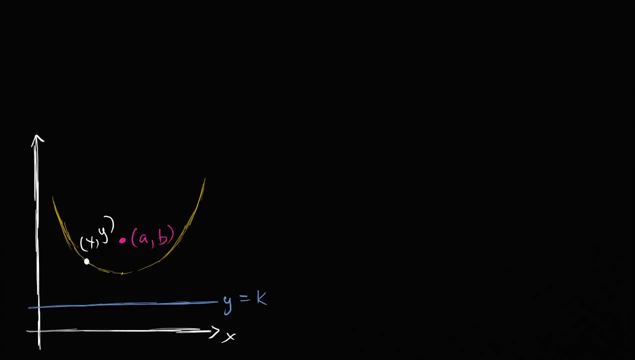 it has to be equidistant to its focus and its directrix. So what does that mean? That means that the distance to the directrix, which I'm drawing here in blue, has to be the same as the distance to the focus. 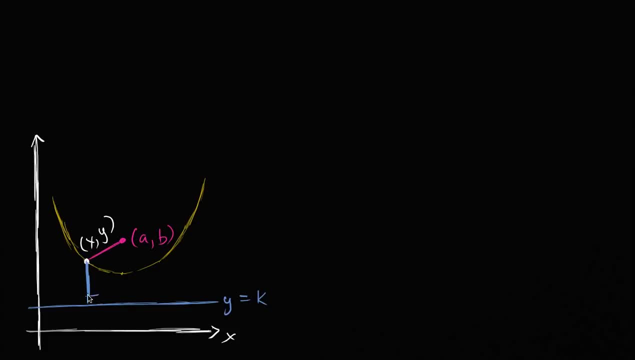 which I am drawing in magenta, And when we take the distance to the directrix, we literally just drop a perpendicular. I guess you could say That's going to be the shortest distance to that line. And then when we the distance to the focus, 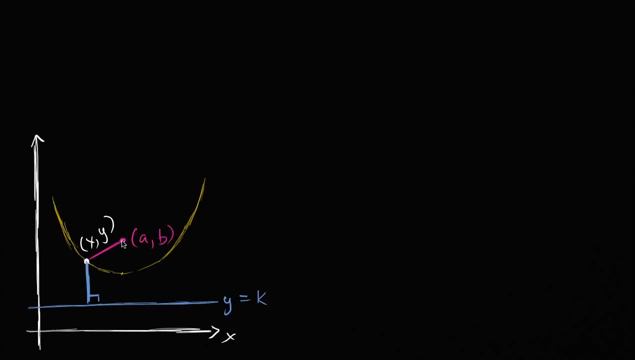 well, we see that's at a bit of an angle and we might have to use the distance formula, which is really just the Pythagorean theorem. So let's do that. This distance has to be the same as that distance. So what's this blue distance? 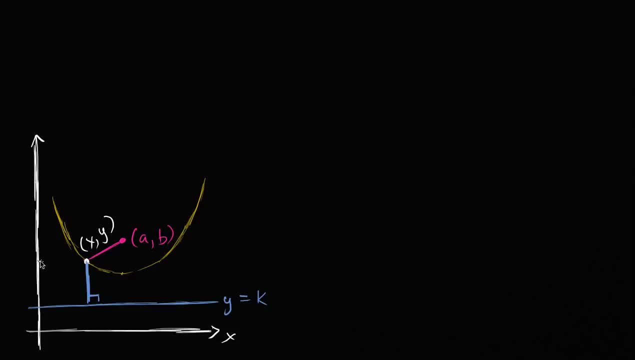 Well, that's just going to be our change in y. It's going to be this: y minus k. It's just this distance, So it's going to be y minus k. Now we have to be careful The way I've just drawn it. yes, y is greater than k. 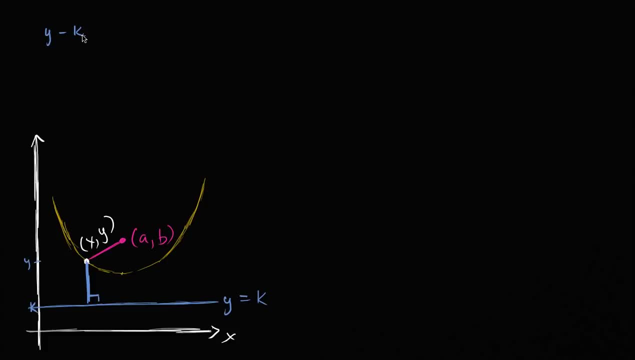 so this is going to give us a positive value And you need a non-negative value. You need a value if you're talking about distances- But there are- you can definitely have a parabola where the y coordinate of the focus is lower than the y coordinate of the directrix. 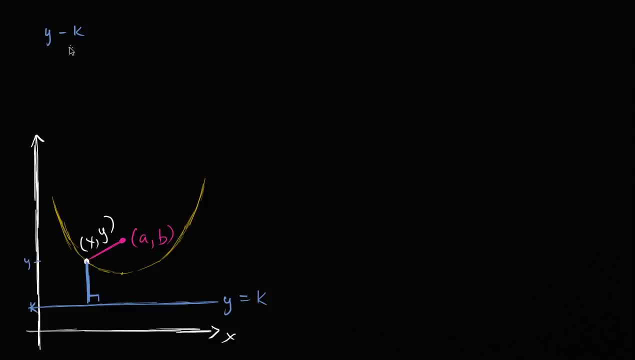 in which case this would be negative. So what we really want is the absolute value of this, or you could say we could square it, and then we could take the square root, the principal root, which would be equivalent to taking the absolute value of y minus k. 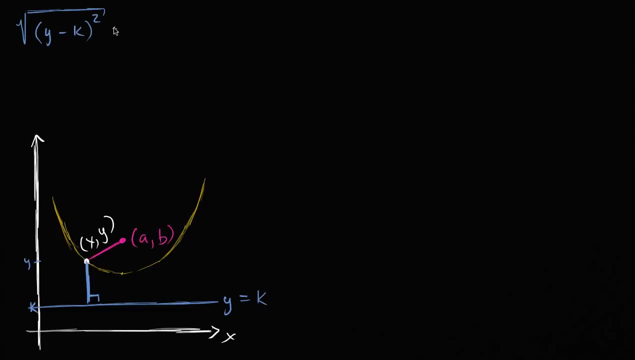 So that's this distance right over here, And by the definition of a parabola, in order for x comma y to be sitting on the parabola, that distance needs to be the same as the distance from x comma y to a comma b to the focus. 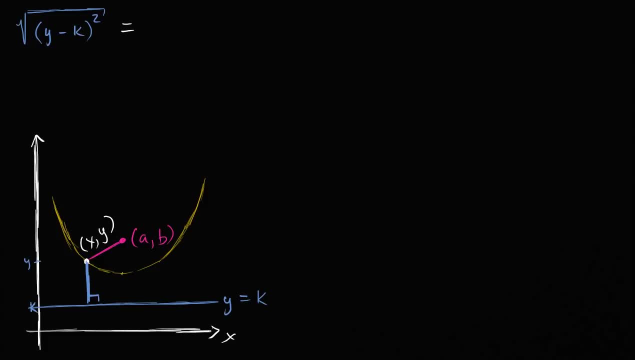 So what's that going to be? Well, we just apply the distance formula or really just the Pythagorean theorem. It's going to be our change in x. so x minus a squared, plus the change in y, y minus b squared, and the square root of that whole thing. 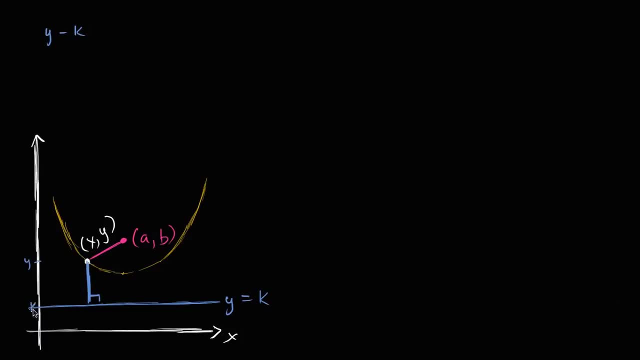 The way I've just drawn it, yes, y is greater than k, so this is going to give us a positive value, and you need a non-negative value, if you're talking about distances. 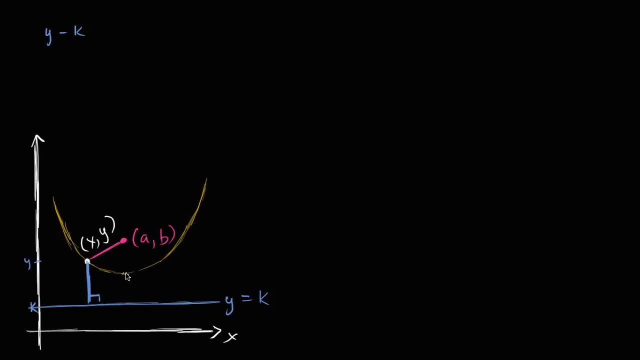 But there are, you can definitely have a parabola where the y coordinate of the focus is lower than the y coordinate of the directrix, in which case this would be negative. So what we really want is the absolute value of this, or you could say, we could square it, and then we could take the square root, the principal root, which would be equivalent to taking the absolute value of y minus k. 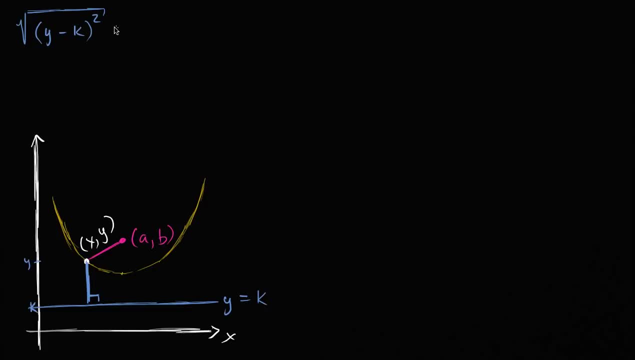 So that's this distance right over here. And by the definition of a parabola, in order for x comma y to be sitting on the parabola, that distance needs to be the same as the distance from x comma y to a comma b, to the focus. 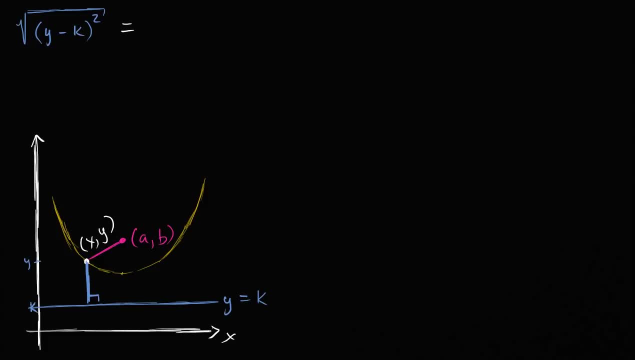 So what's that going to be? Well, we just apply the distance formula, or really just the Pythagorean theorem. 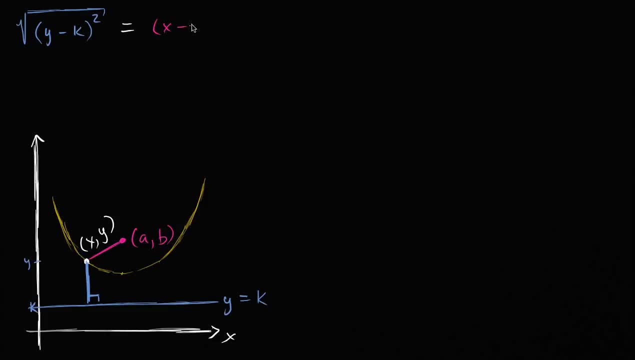 It's going to be our change in x, so x minus a squared, plus the change in y, y minus b squared, and the square root of that whole thing. The square root of all of that business. Now, this right over here is an equation of a parabola. It doesn't look like it. It looks really hairy, but it is the equation of a parabola. And to show you that, we just have to simplify this. And if you get inspired, 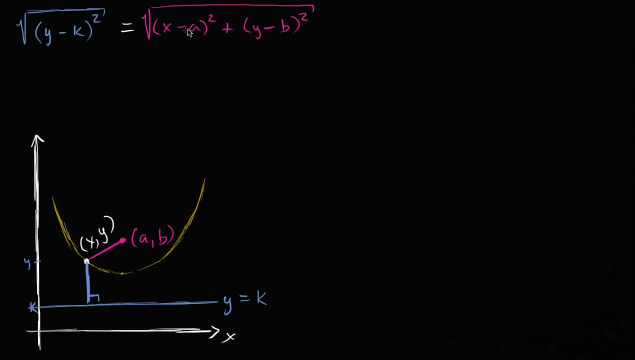 I encourage you to try to simplify this on your own. It's just going to be a little bit of hairy algebra, but it really is not too bad. 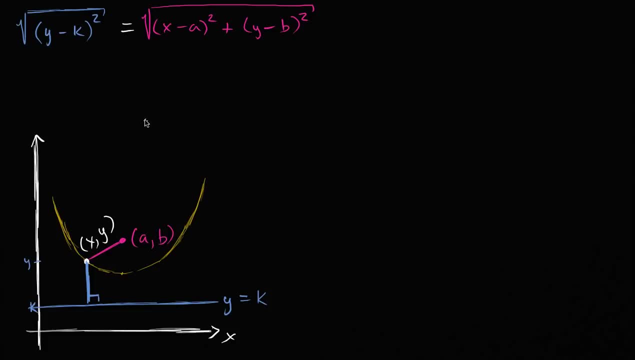 You're going to get an equation for a parabola that you might recognize, and it's going to be in terms of kind of a general focus, a comma b, and a general directrix, y equals k. So let's do that. 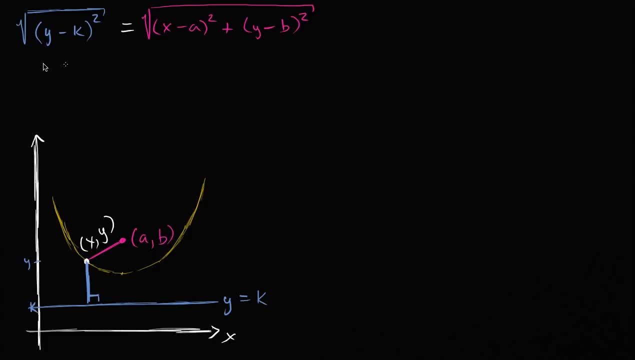 is let's just square both sides so we get rid of the radicals. So if you square both sides, on the left-hand side, you're going to get y minus k squared. You're going to get y minus k squared is equal to x minus a squared plus y minus b squared. Fair enough. 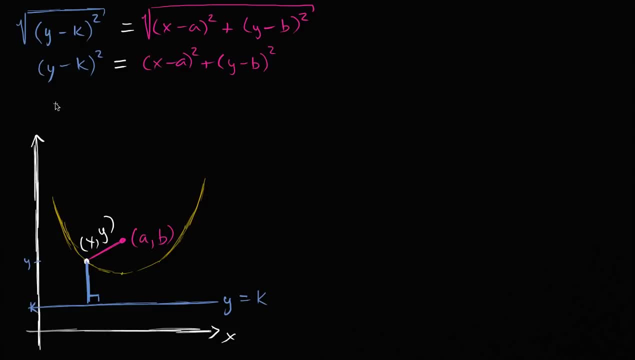 Now, what I want to do is I just want to end up with just a y on the left-hand side and just x's, a's, b's, and k's on the right-hand side. 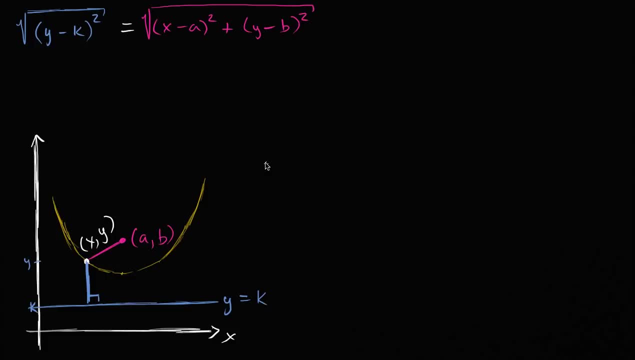 The square root of all of that business. Now, this right over here is an equation of a parabola. It doesn't look like it, It looks really hairy, but it is the equation of a parabola. And to show you that, we just have to simplify this. 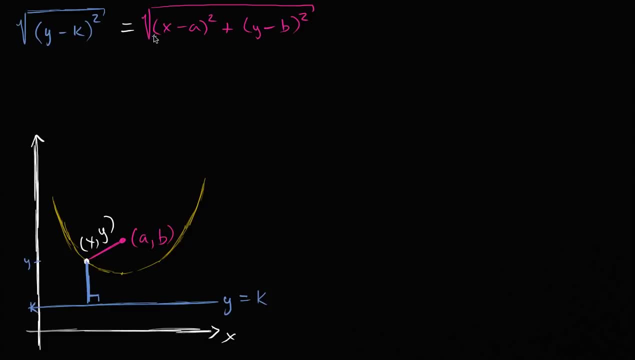 And if you get inspired, I encourage you to try to simplify this on your own. It's just going to be a little bit of hairy algebra, but it really is not too bad. You're going to get an equation for a parabola. 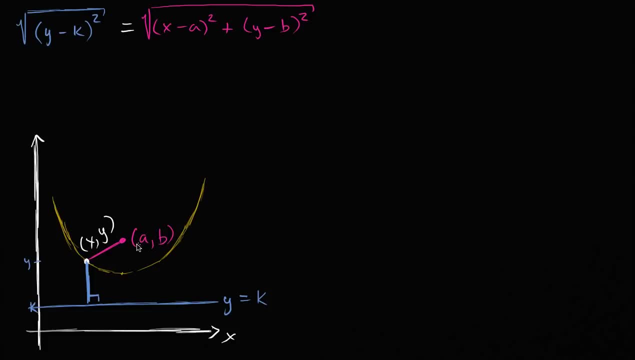 that you might recognize, and it's going to be in terms of kind of a general focus a, comma b and a general directrix. y equals k, So let's do that. So the simplest thing to start here is: let's just square both sides. 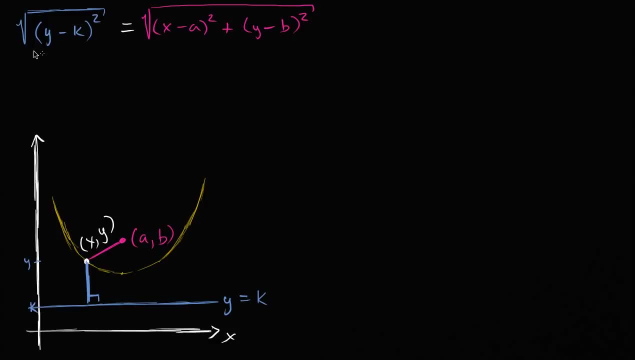 so we get rid of the radicals. So if you square both sides, on the left-hand side you're going to get: y minus k squared is equal to x minus a squared, plus y minus b squared. Fair enough, Now what I want to do is I just want to end up. 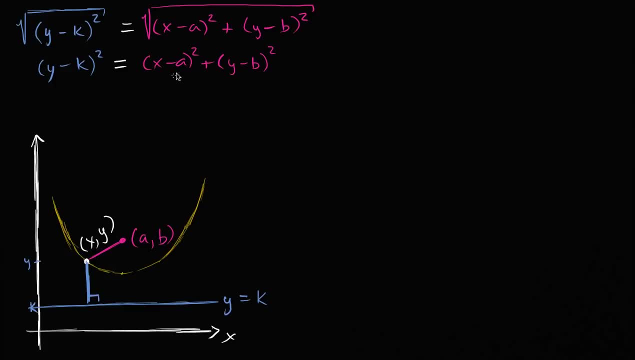 with just a y on the left-hand side and just x's, a's, b's and k's on the right-hand side. So the first thing I might want to do is let's expand each of these expressions that involve with y. 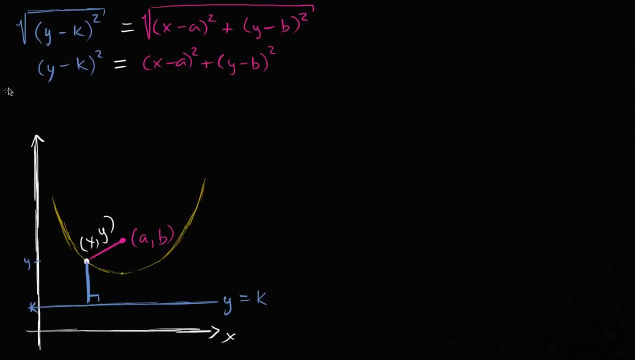 So this blue one on the left-hand side, that is going to be y squared minus 2yk plus k squared and that is going to be equal to. I'm going to keep this first one the same. so it's going to be x minus a squared. 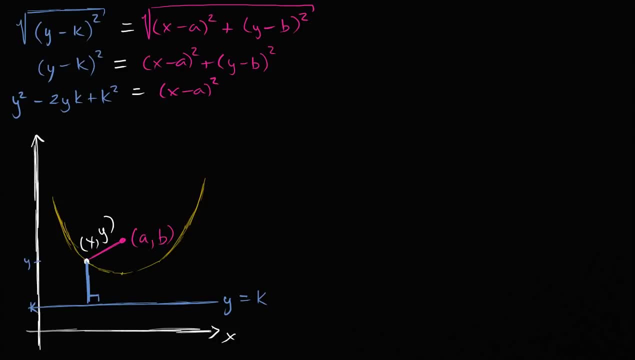 and now let me expand. let me expand. I'm going to find a color. expand this in green. So, plus y squared minus 2yb, plus b squared, All I did is I multiplied y minus b times y minus b. Now let's see if we can simplify things. 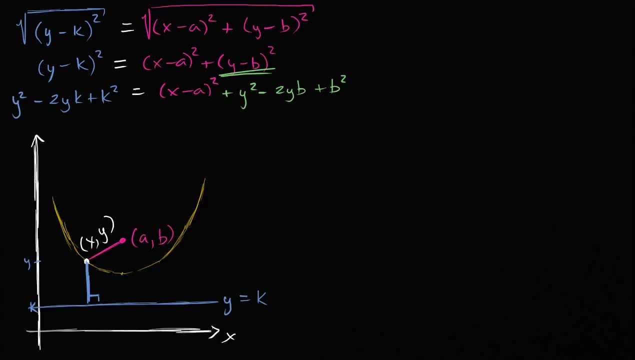 So I have a y squared on the left, I have a y squared on the right. Well, if I subtract y squared from both sides, so I can do that. Well, that simplified things a little bit, And now I can. I can. let's see what I can do. 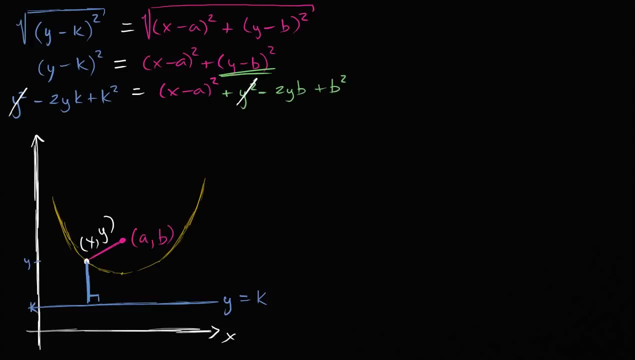 Well, let's get the k squared on this side. So let's subtract k squared from both sides. So subtract k squared, Subtract k squared from both sides. So that's going to get rid of it on the left-hand side. And now let's add 2yb to both sides. 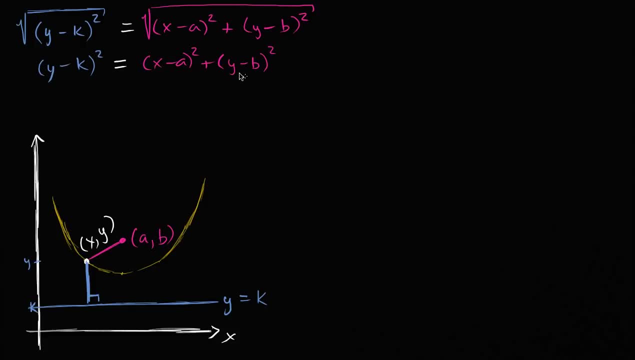 So the first thing I might want to do is let's expand each of these expressions that involve with y. So this blue one on the left-hand side, 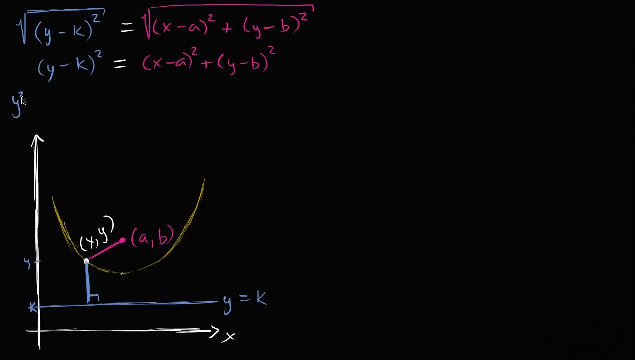 that is going to be y squared minus 2yk plus k squared, and that is going to be equal to, I'm going to keep this first one the same, so it's going to be x minus a squared, and now let me expand, let me expand, I'm going to find a color, expand this. 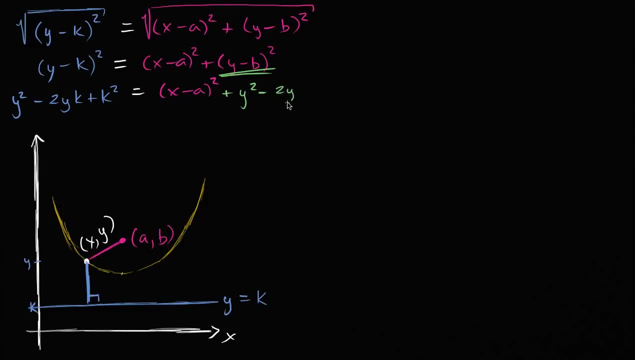 It's going to be green, so plus y squared minus 2yb plus b squared. 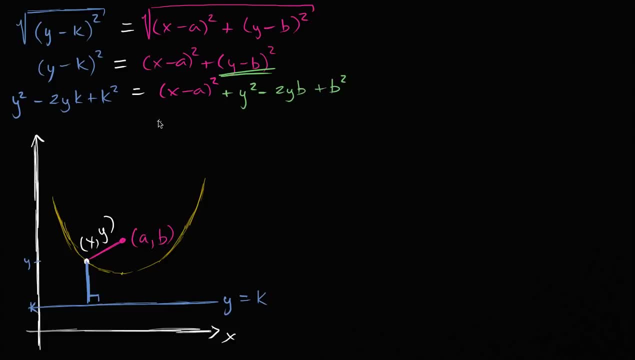 All I did is I multiplied y minus b times y minus b. Now let's see if we can simplify things. So I have a y squared on the left, I have a y squared on the right. Well, if I subtract y squared from both sides, so I can do that. 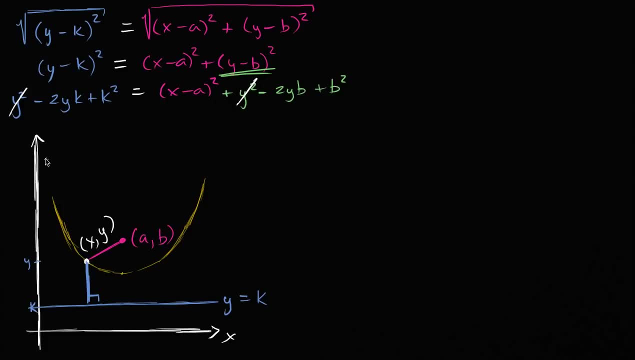 Well, that simplified things a little bit. And now I can, I can, let's see what I can do. Well, let's get the k squared on this side. So let's subtract k squared from both sides. So subtract k squared, subtract k squared from both sides, so that's going to get rid of it on the left-hand side. And now let's add 2yb to both sides, so we have all the y's on the left-hand side. 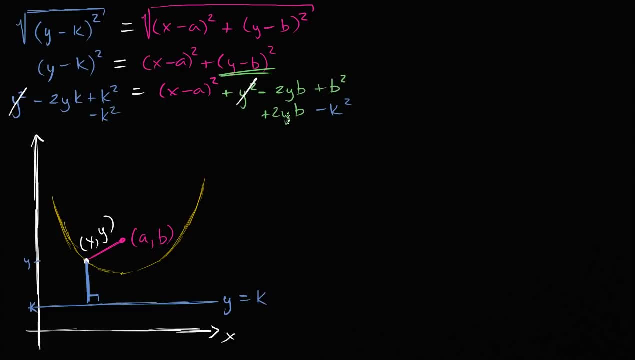 So plus 2yb, that's going to move, that's going to give us a 2yb on the left-hand side, 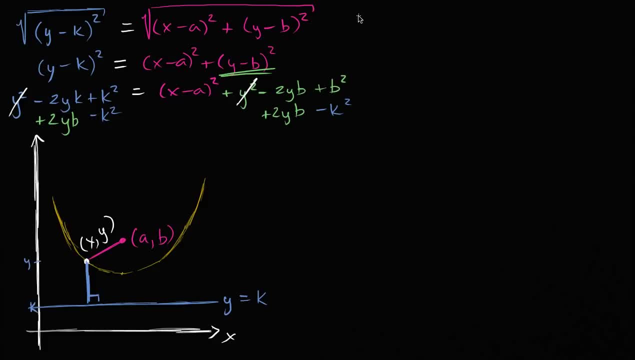 So what is this going to be equal to? I'm starting to run into my graph, so let me give myself a little bit more real estate over here. 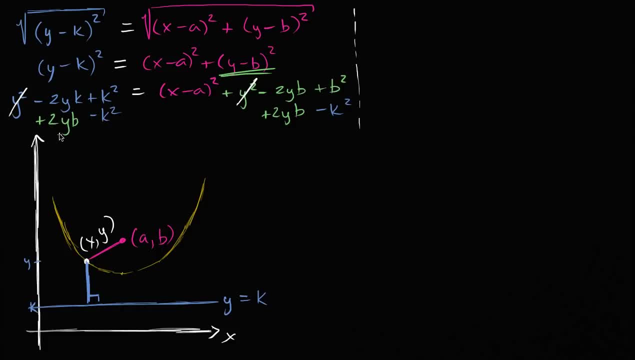 So on the left-hand side, what am I going to have? This is the same thing as 2yb minus 2yk, which is the same thing, actually, let me just write that down. That's going to be 2y, 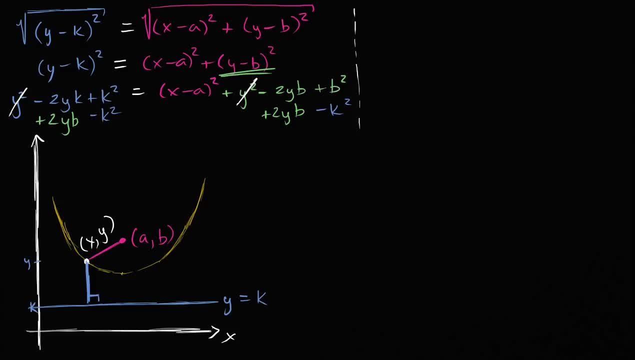 do it in green. Actually, well, yeah, why not green? That's going to be, actually, let me start a new color. 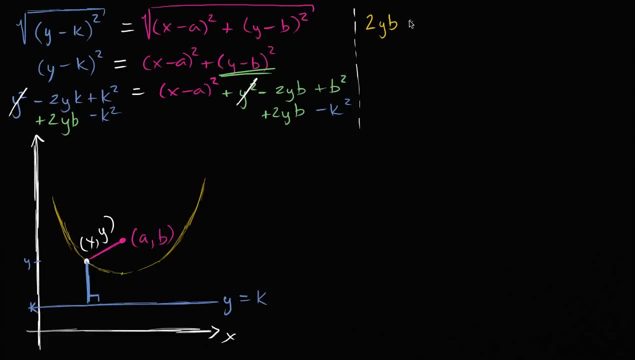 That's going to be 2yb minus 2yk. You can focus, you can factor out a 2y, and it's going to be 2y times b minus k. So let's do that. 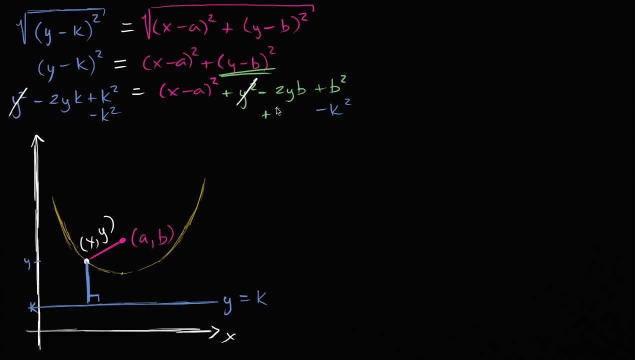 so we have all the y's on the left-hand side. So plus 2yb, that's going to move. that's going to give us a 2yb on the left-hand side plus 2yb. So what is this going to be equal to? 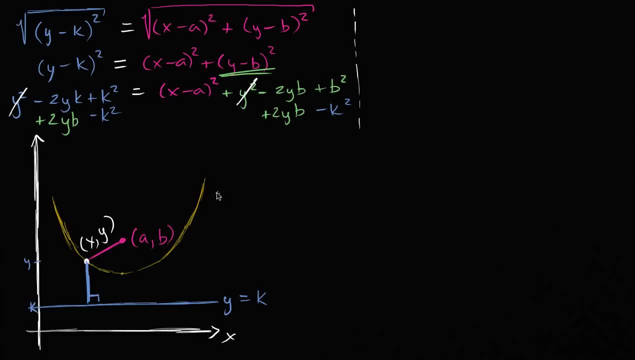 I'm starting to run into my graph, so let me give myself a little bit more real estate over here. So, on the left-hand side, what am I going to have? This is the same thing as 2yb minus 2yk. 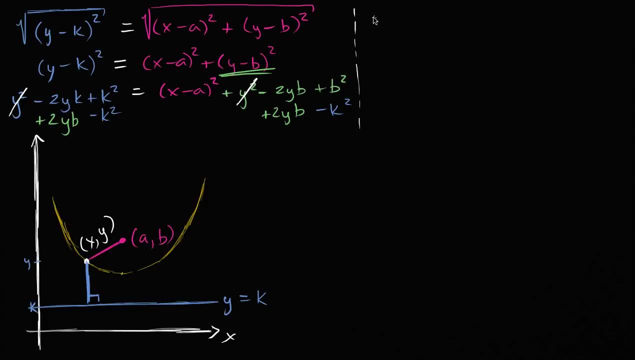 which is the same thing actually. let me just write that down. That's going to be 2y. do it in green Actually. well, yeah, why not green? That's going to be actually. let me start a new color. 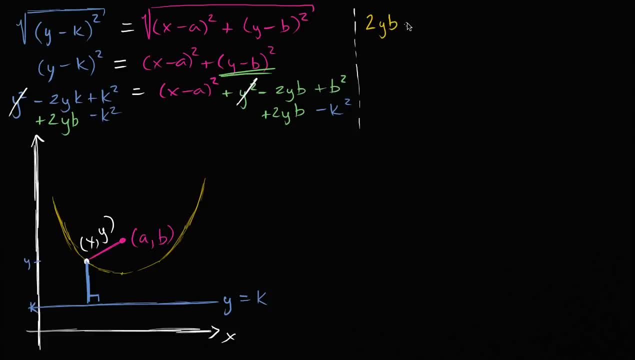 That's going to be 2yb minus 2yk. You can focus, you can factor out a, 2y and it's going to be 2y times b minus k. So let's do that, So we could write this as 2,. 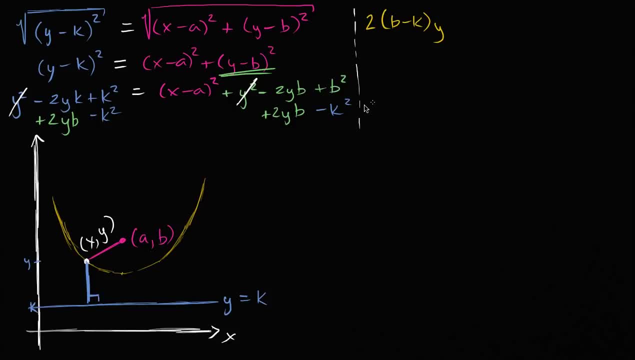 or we could write it 2 times: b minus ky. if you factor out a, 2 and a, y, So that's the left-hand side, so that's that piece right over there. These things cancel out. Now on our right-hand side, 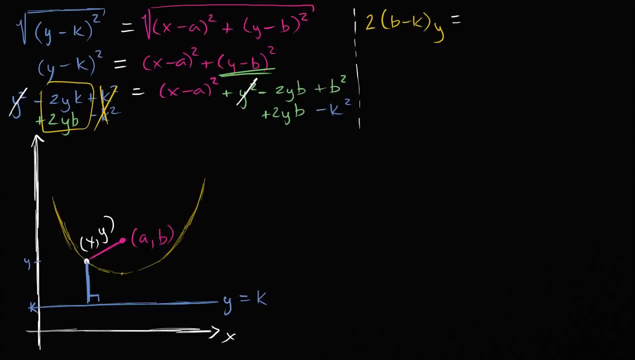 I promised you a little bit of hairy algebra, so hopefully you see that I'm delivering on that promise. On the right-hand side you have x minus a squared, and then let's see these characters cancel out and you're left with b squared minus ky. 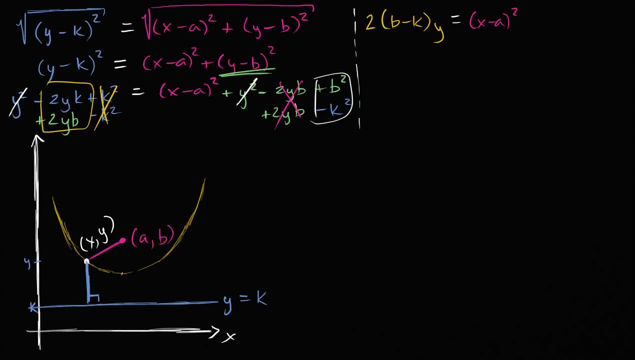 So these two are going to be b squared minus k squared, plus b squared minus k squared. Now I said all I want is a y on the left-hand side. so let's divide everything by 2 times b minus k. So let's divide everything times 2 times b minus k. 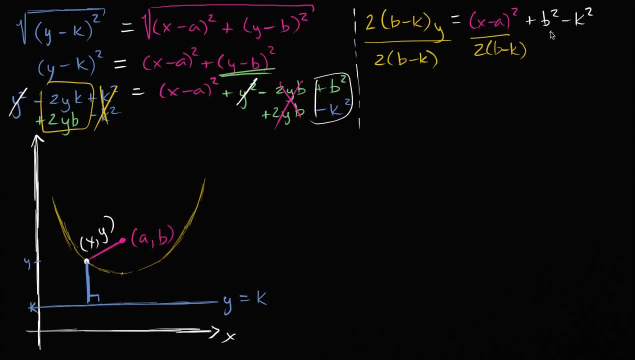 So 2 times b minus k, and I'm actually going to divide this whole thing by 2 times b minus k. Now, obviously, on the left-hand side, this all cancels out. You're left with just a y, and then it's going to be y equals. 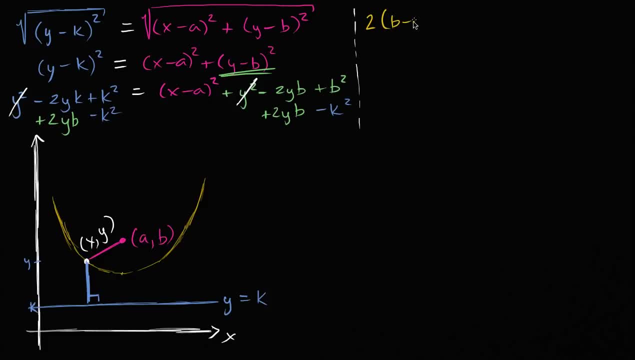 So we could write this as 2, or we could write it 2 times b minus ky, 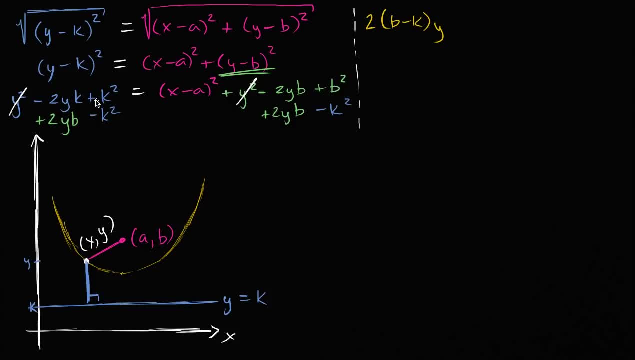 if you factor out a 2 and a y. So that's the left-hand side. So that's that piece right over there. 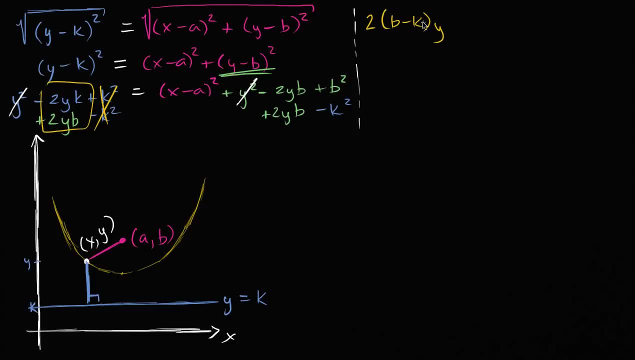 These things cancel out. Now on our right-hand side, 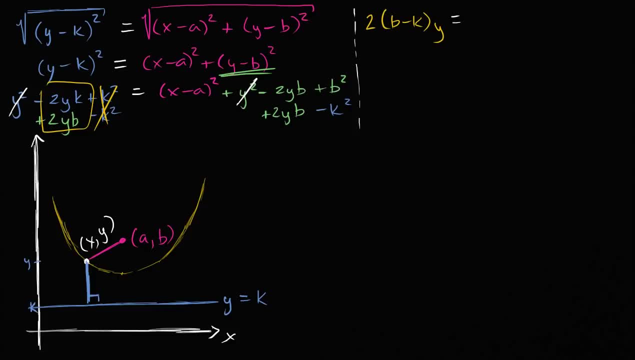 I promised you a little bit of hairy algebra, so hopefully you see that I'm delivering on that promise. 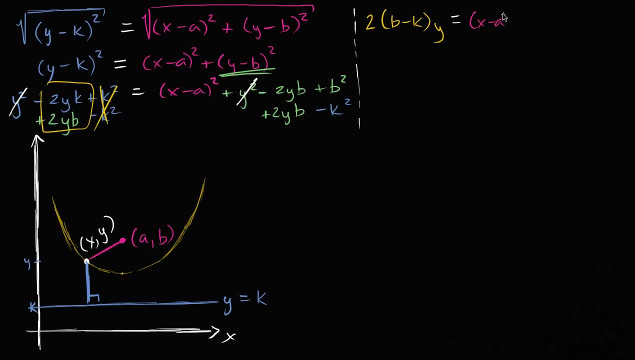 On the right-hand side, you have x minus a squared, and then, let's see, these characters cancel out, and you're left with b squared, minus k squared. So these two are going to be b squared minus k squared, plus b squared minus k squared. 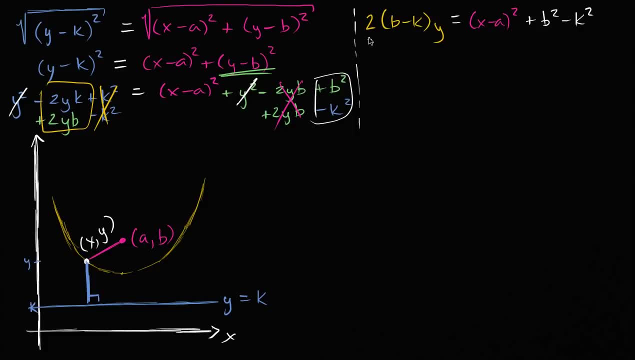 Now, I said all I want is a y on the left-hand side, so let's divide everything by 2 times b minus k. So let's divide everything times 2 times b minus k. So 2 times b minus k, and I'm actually going to divide this whole thing by 2 times b minus k. Now, obviously, on the left-hand side, this all cancels out. You're left with just a y, and then it's going to be y equals, y is equal to 1 over 2 times b minus k. 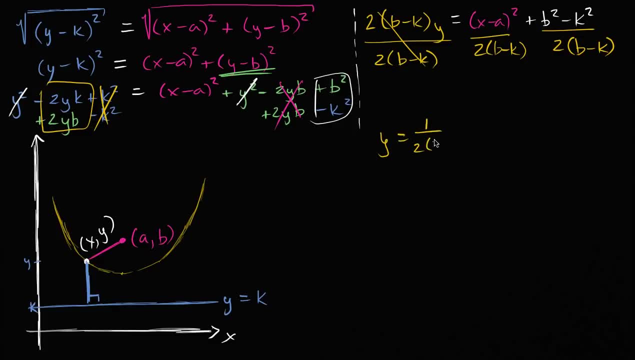 y is equal to 1 over 2 times b minus k. and notice, b minus k is the difference between the y-coordinate of the focus and the y-coordinate, I guess you could say, of the line. y equals k, So it's 1 over 2 times that. 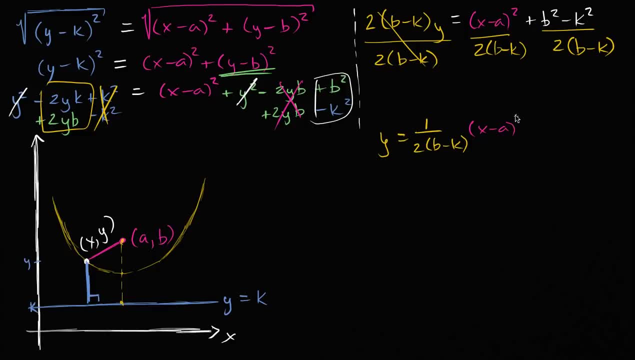 times x minus a squared. So if you knew what b minus k are, this would just simplify to some number, some number that's being multiplied times x minus a squared. So hopefully this is starting to look like the parabolas that you remember. 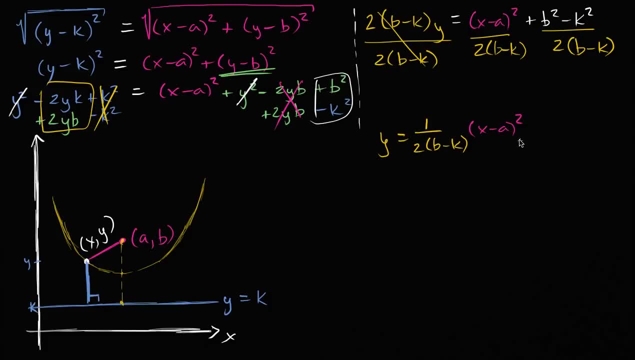 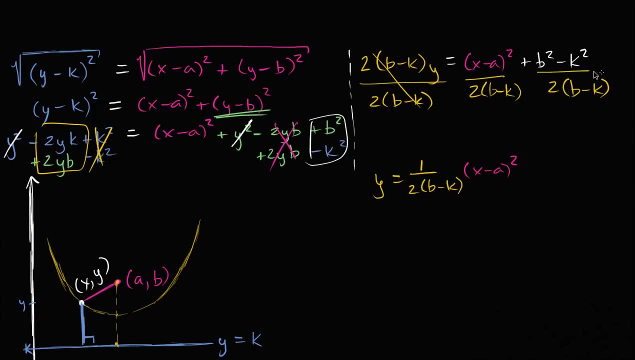 from your childhood. if you do remember parabolas from your childhood, All right. so then let's see if we could simplify this thing on the right and you might recognize b squared minus k squared. that's the difference of squares, That's the same thing as. 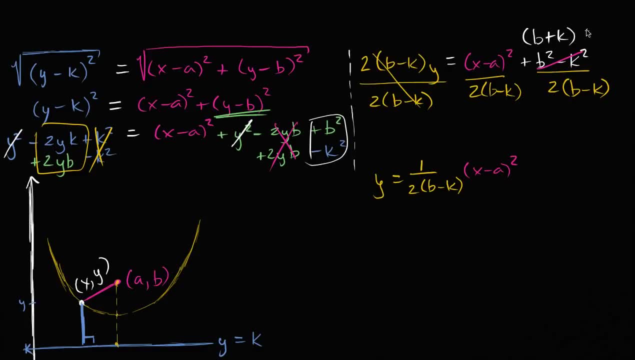 that's the same thing as b plus k times b minus k, times b whoops, times b minus k. So the b minus k's cancel out and we are just left with, and we deserve a little bit of a drum roll. 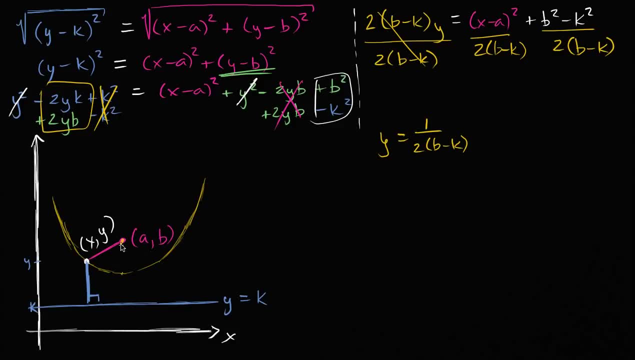 And notice, b minus k is the difference between the y-coordinate of the focus and the y-coordinate, I guess you could say, of the line, y equals k. So it's 1 over 2 times that, times x minus a squared, x minus a squared. So if you knew what b minus k was, whoa, are, this would just simplify to some number. 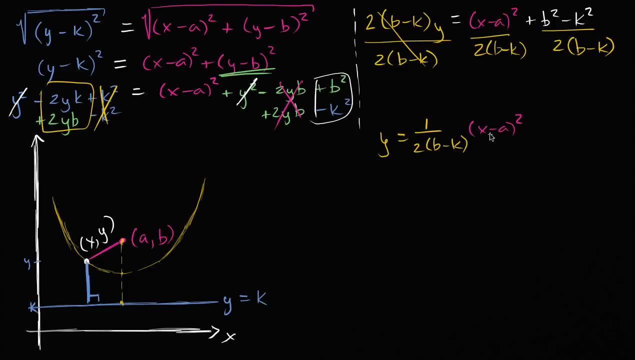 Some number that's being multiplied times x minus a squared. 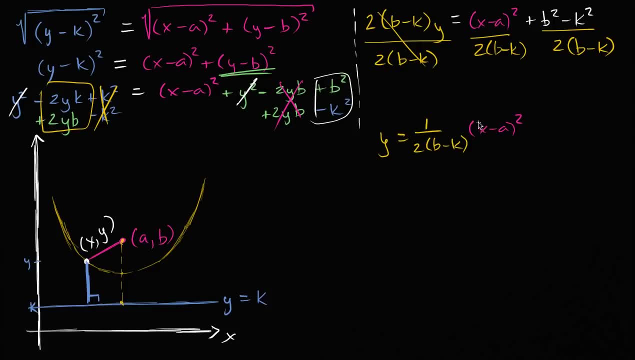 So hopefully this is starting to look like the parabolas that you remember from your childhood. If you do remember parabolas from your childhood. 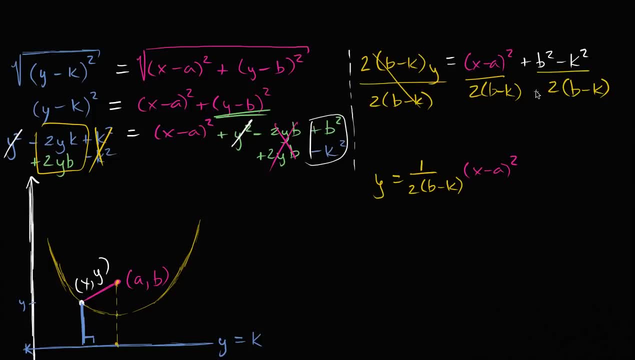 All right, so then let's see if we could simplify this thing on the right, and you might recognize b squared minus k squared, that's the difference of squares. 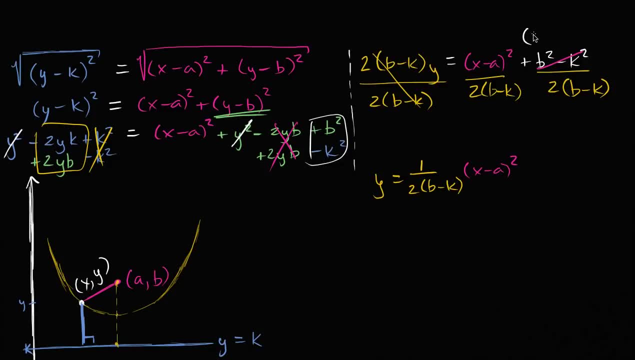 That's the same thing as, that's the same thing as b plus k times b minus k, times b, whoops, times b minus k. So the b minus k's cancel out, and we are just left with, and we deserve a little bit of a drum roll, we're just left with 1 half times b plus k. So there you go. 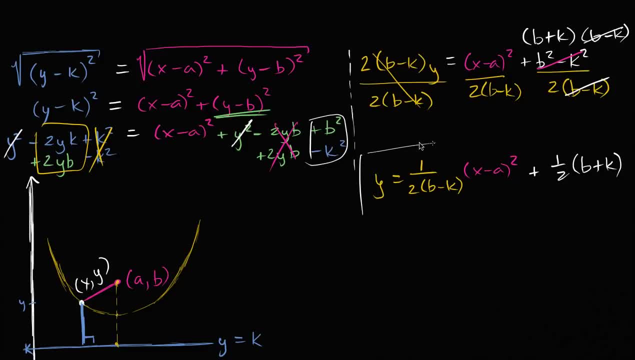 Given a focus at the point a comma b, and a directrix at y equals k, we now know what the formula of the parabola is actually going to be. 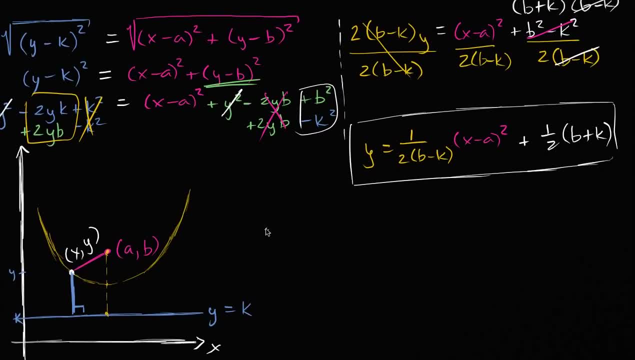 So for example, so for example, if I had a focus, if I had a focus at the point, I don't know, let's say the point 1 comma 2, and I had a directrix, I had a directrix at y, y is equal to, I don't know, let's make it y is equal to negative 1, what would the formula, 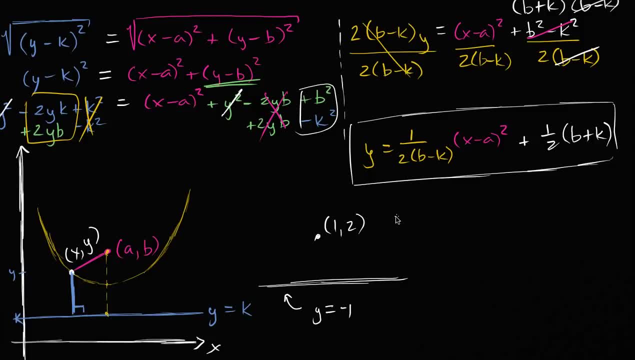 or what would the equation of this parabola be? Well, it would be y is equal to, 1 over 2 times b minus k, so 2 minus negative 1, that's the same thing as 2 plus 1, so that's 2 times, that's just 3, 2 minus negative 1 is 3, times x minus, times x minus 1, whoops, x minus 1 squared, plus 1 half times b plus k. 2 plus negative 1 is 1. So 1. 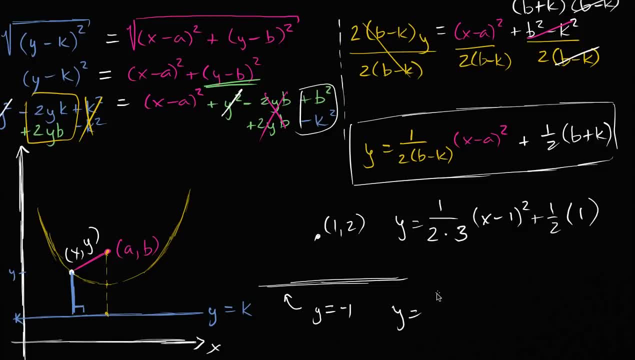 And so what's this going to be? You're going to get y is equal to 1 over 1 sixth x minus 1 squared 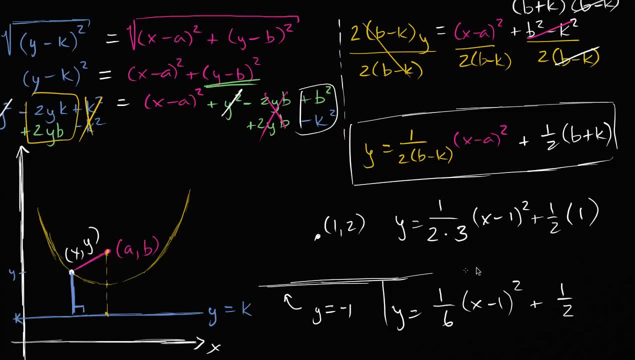 plus 1 half. There you go. 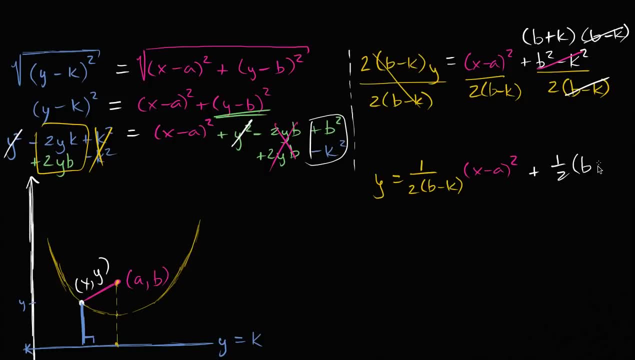 we're just left with 1 half times b plus k. So there you go. Given a focus at the point a, comma b and a directrix at y equals k. we now know what the formula of the parabola is actually going to be. 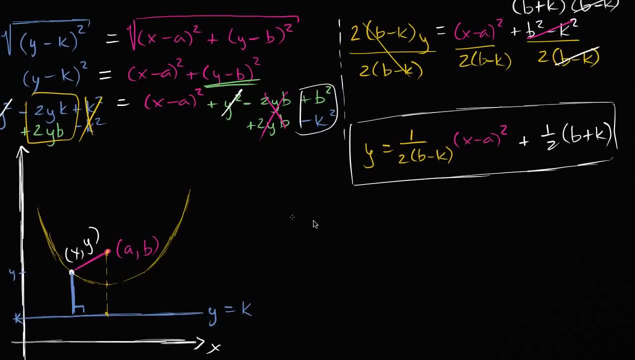 So, for example. so, for example, if I had a focus, if I had a focus at the point I don't know, let's say the point 1, comma 2, and I had a directrix. I had a directrix at y. 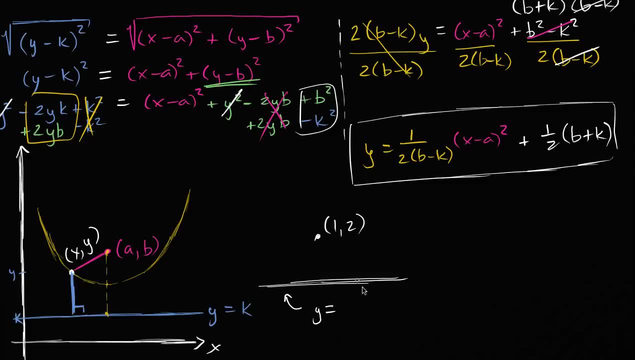 y is equal to. I don't know, let's make it: y is equal to negative 1,. what would the formula or what would the equation of this parabola be? Well, it would be: y is equal to 1 over. 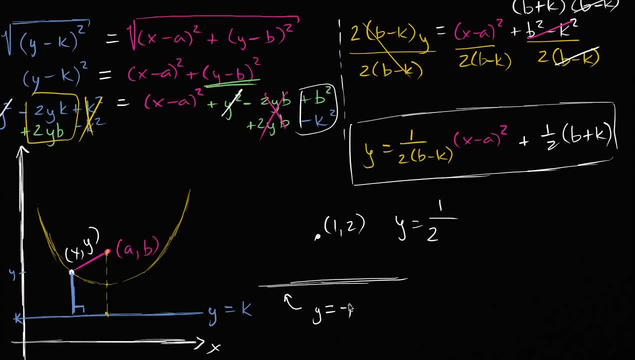 2 times b minus k, so 2 minus negative 1, that's the same thing as 2 plus 1, so that's 2 times that's just 3,. 2 minus negative 1 is 3, times x minus. 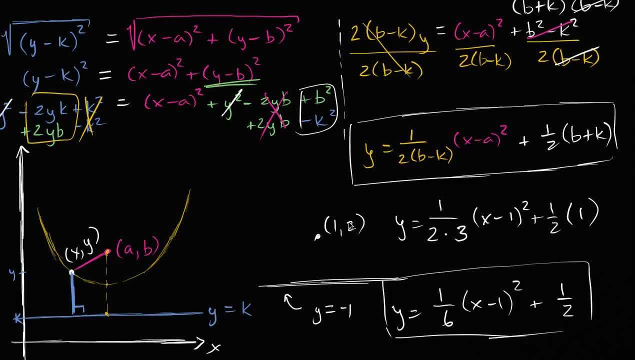 That is the parabola with a focus at 1 comma 2 and a directrix at y equals negative 1. Fascinating.